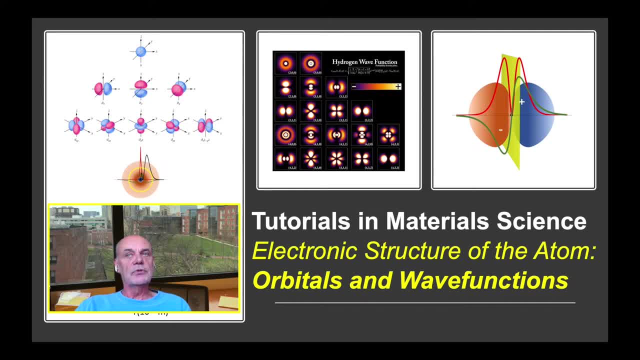 function as well as its sine, which we already know is the amplitude of the wave function. In this first video we begin with a general overview of quantum numbers and then talk about the phase and we'll get into the probability density, which is psi squared. We then focus on 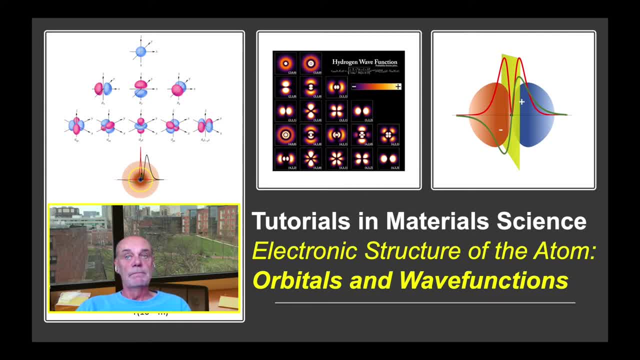 visualizing the wave functions using orbital pictures, and the second and third videos explain how we can represent the radial and the angular components of the wave functions in separate pictures. The last video will then focus on the energy states of electrons in the atomic orbitals. 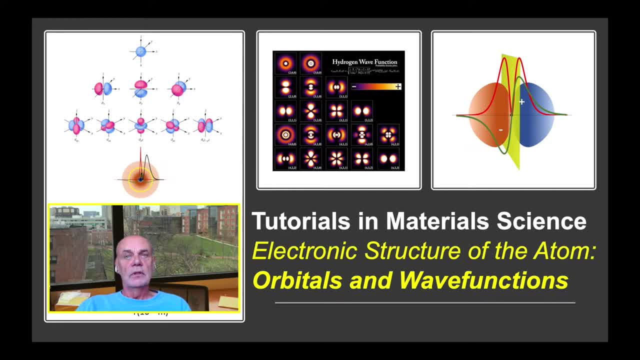 How they change across the periodic table and how those changes in turn can be used to understand the periodic trends in atom size and electronegativity, which are critical in predicting the type of bonding exhibited by a material in the solid state. I hope you'll find. 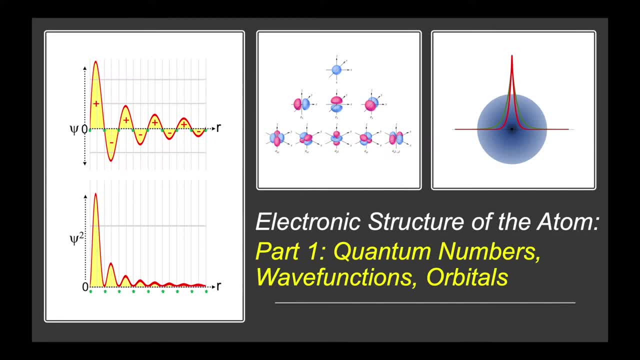 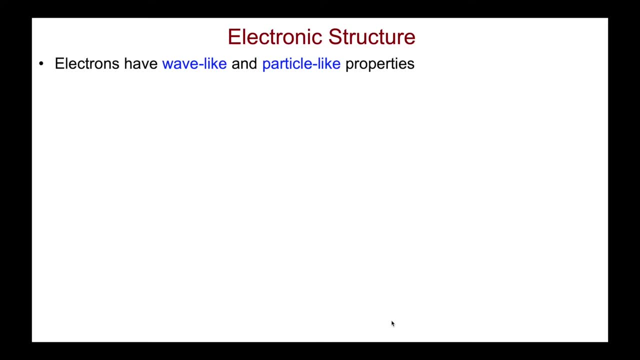 these videos useful to you. Let's just begin with a short overview of what I'm hoping everyone has seen before in freshman chemistry. So electrons have wave-like and particle-like properties. We're going to focus on the wave-like properties here. They diffract like light and they also occupy orbitals, and here are some of the orbital. 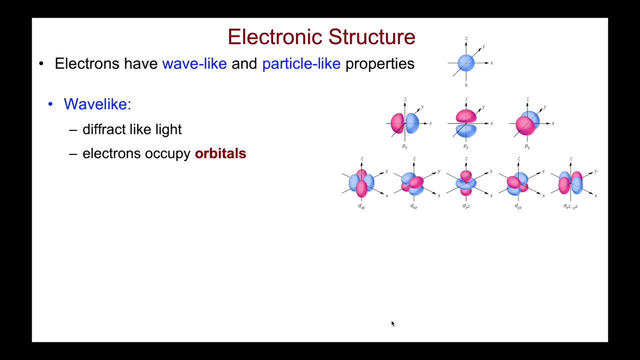 pictures shown on the right: The s, the p's, the d's. that we'll get into later, but you should again have seen before. Orbitals represent the space in an atom occupied by an electron. That space is described by wave functions and the wave function is called psi. Psi has amplitude, it has nodes and phase. 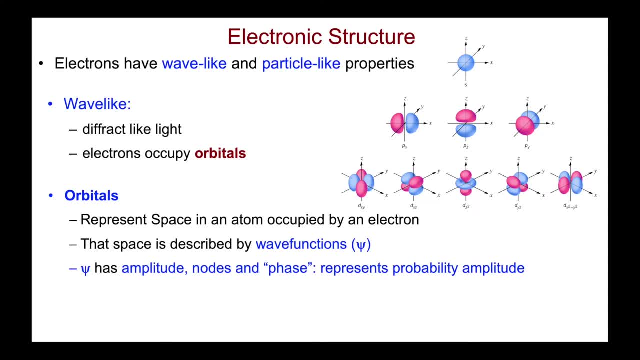 and it represents the probability amplitude of the electron. Psi squared represents the probability density, probability of finding the location of the electron in a given point or at a given radius of that orbital, The size, the shape and the orientation of that probability, density. and 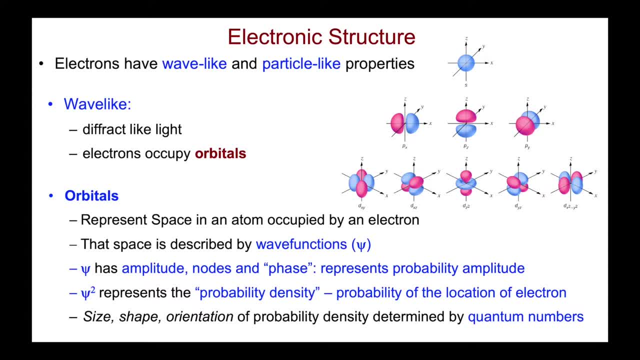 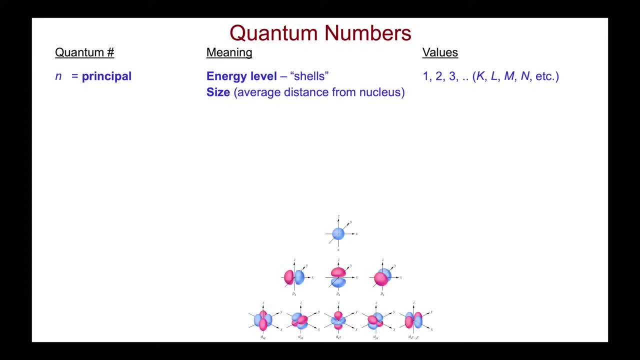 of the wave function itself is determined by quantum numbers which, again, you should have seen before and we'll very briefly review here. First the principal quantum number n. This really dictates the energy level, but not entirely, as we'll see later. So this represents the size or the average distance from the nucleus of the electron in. 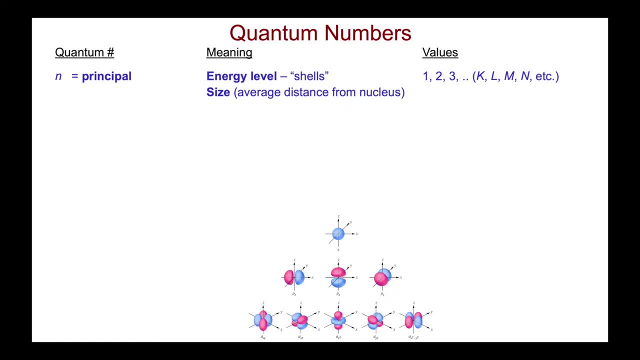 the orbital. It can have values of 1,, 2,, 3, etc. which sometimes are called the K, L, M and N shell. The next important quantum number is the L, the orbital quantum number, sometimes called the azimuthal quantum number. L represents, or its meaning is, the shape of the sub-shells. 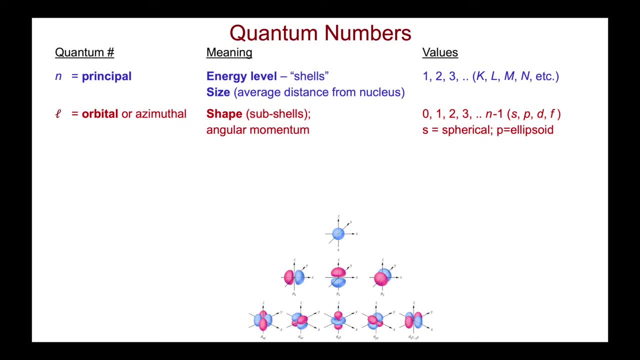 And we'll see also later. it represents the angular momentum. L can take on values of 0,, 1,, 2,, 3, up to a maximum of n minus 1.. And these numbers are usually replaced by letters. So for L is 0, we call that the s-orbital L is 1,, the p-orbital L is 2, the d-orbitals 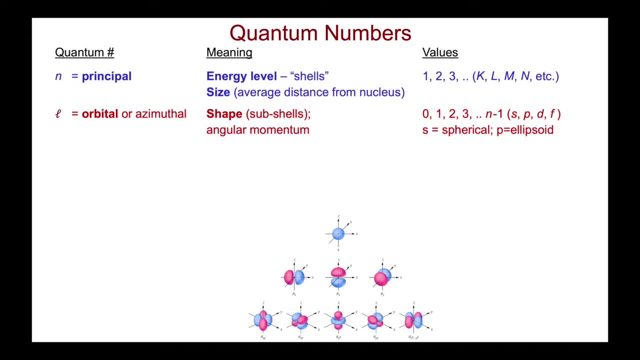 L is 3, the f-orbitals, etc. With respect to the shape, then, for the L equals 0, s-orbitals- they're spherical, The p-orbitals are ellipsoids. M sub L is the magnetic quantum number. This actually represents the orientation and the 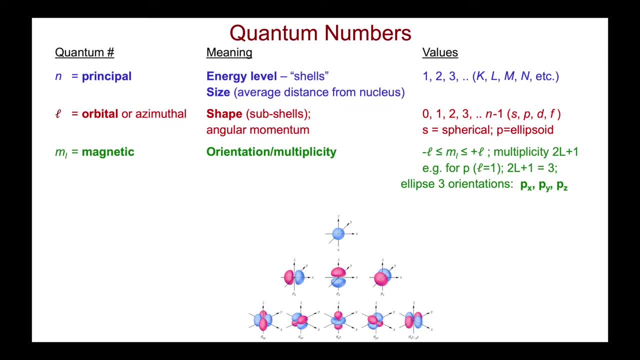 multiplicity of the orbitals M sub L can range in values from plus L to minus L, and its multiplicity is 2L plus 1.. Let's take a simple example for the p-orbital which has L equal to 1.. 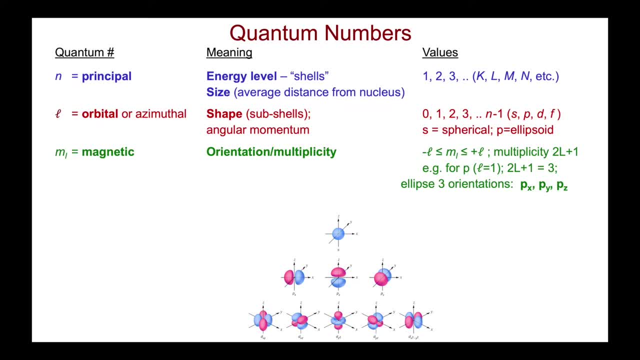 And so the values of M sub L could be plus 1,, 0 and minus 1.. And so there's three possible p-orbitals: The p-x, the p-y and the p-z. The p-x, the p-y and the p-z. 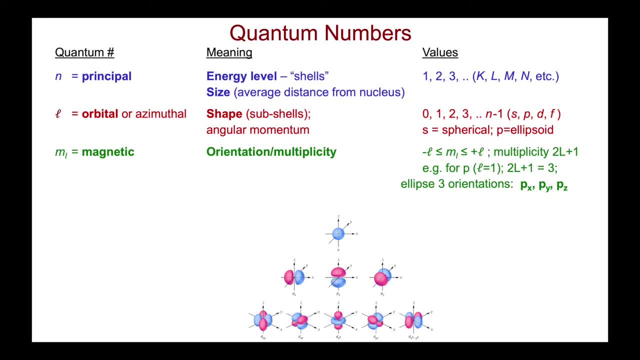 And so this ellipsoid has three possible orientations associated with those major Cartesian axes. And finally, we have the spin quantum number M sub s. This is not so much a property of an orbital but the property of an electron. It could have spin up or spin down, which in turn takes values of plus a half or minus a half. 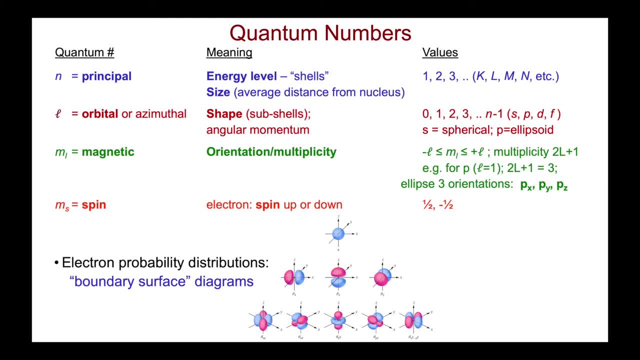 And so in the end from all of these quantum numbers we can sketch the orbitals and their orientations using boundary surface diagrams, And so the sketches here really represent the electron probability distributions, both their radial extent and their angular dependence. So that was just a brief overview of quantum numbers and wave functions, But for the rest of this model we'll just go along with the rest of the data. 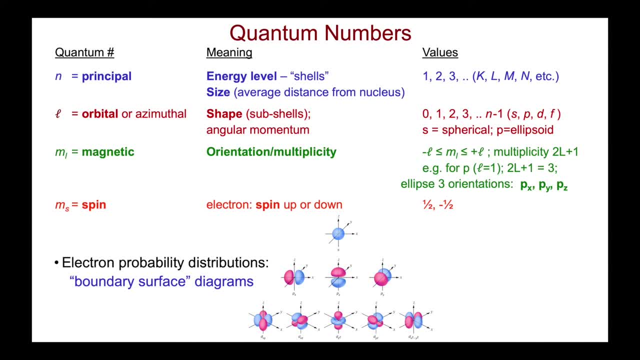 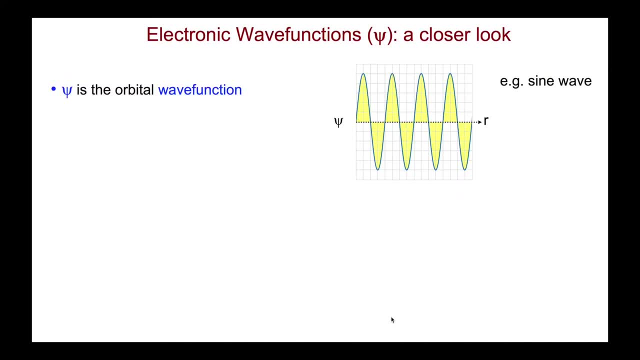 we'll go into things a little bit more slowly and with a little bit more detail. So let's take a closer look at the electronic wave functions. Symbol is psi. So psi is the wave function of the orbital and we're going to see the 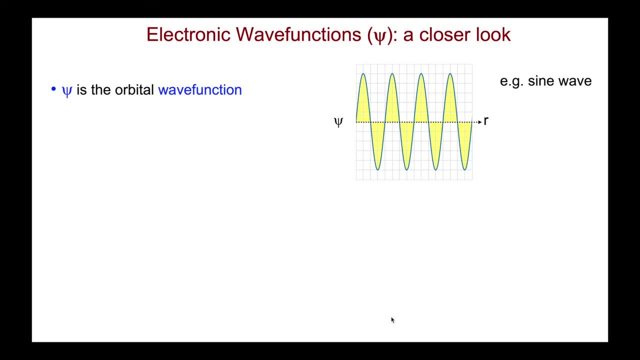 equations, for it can be a little bit intimidating. but for now let's just consider a regular sine wave. Well, I think we're comfortable with the fact that a wave has amplitude and phase, or the sine of the wave function. So in this case the wave function is positive. 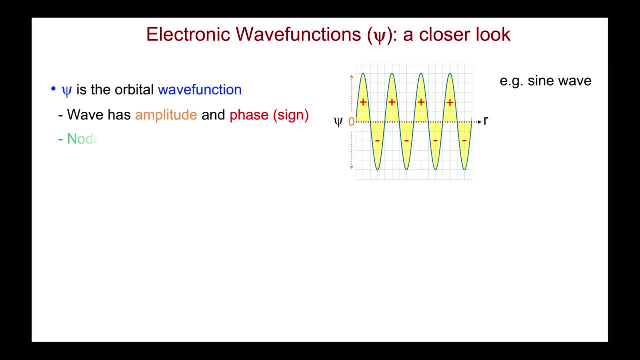 here and negative down here. This particular wave wave function also has nodes. Nodes are simply where the wave function itself has no amplitude, such as these points highlighted here. And at a node it changes sign. It goes from a positive sign to a negative sign. So the positions, 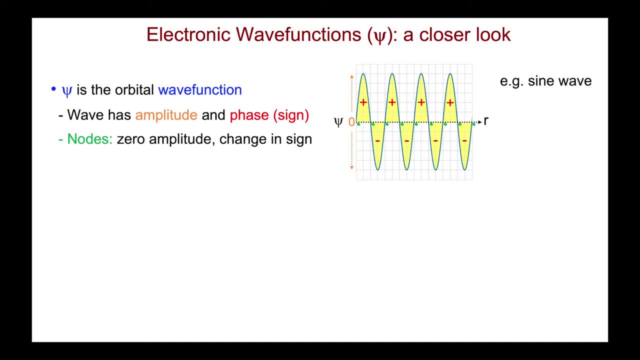 of the nodes are also of particular importance. Again, that's where the wave function has no amplitude. Psi squared is the probability, density, the likelihood of finding the electron at any particular position. It is the square of the wave function. So here I've taken my sine wave, squared it and of course all. 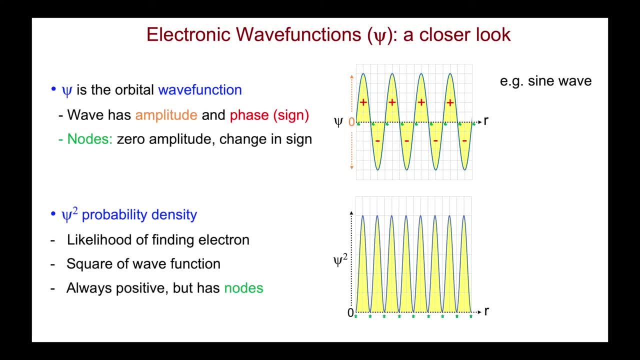 of the resultant amplitudes are positive, But it still has nodes. So it we note here. In this case, psi squared is zero. What does that really mean? That means there is no chance of having any amplitude of that particular value of r. And when we relate that 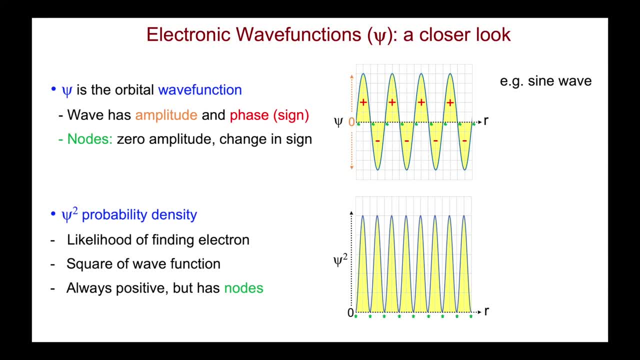 to an electron. it means the electron has absolutely no chance of being at that position. Where is it? It could be anywhere else, represented by the different probabilities, But the nodes are significant because there we know it has no amplitude, no probability density. 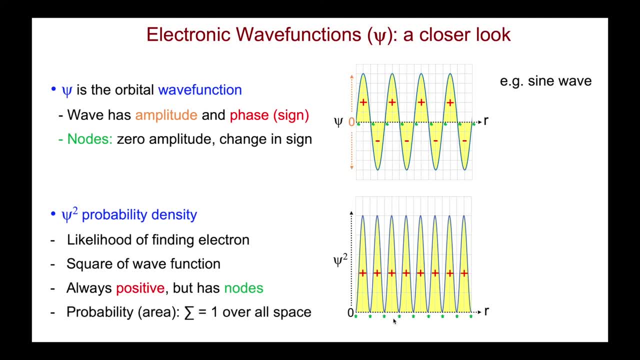 We do know, however, that the sum of the probability over all space must be one, So the sum of psi squared equals one, meaning that we've got a hundred percent probability of finding the electron somewhere. We just don't know exactly where, But again, we do know where it is not. 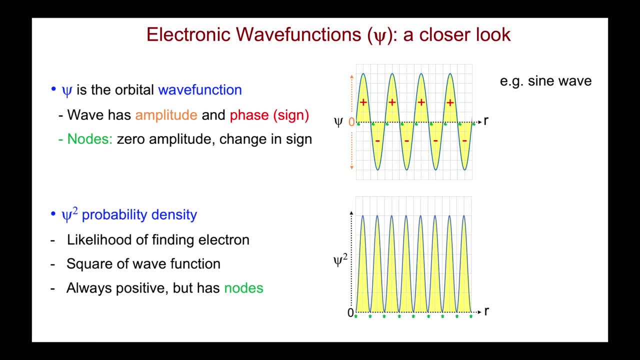 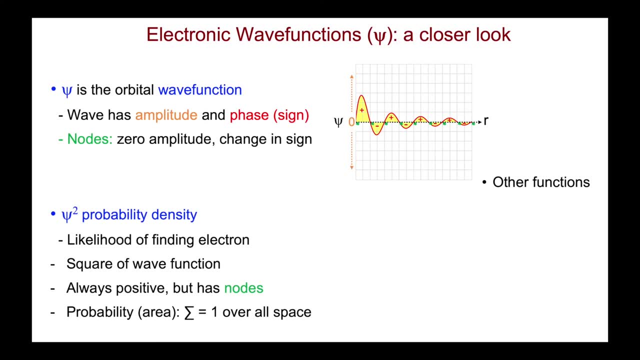 Well, this is just a simple sine wave. We'd consider a slightly more complicated function. This is the damped sine wave. The details don't matter. But again we see the wave function has amplitude, It has nodes, It changes at a node from a positive sign to a negative sign. 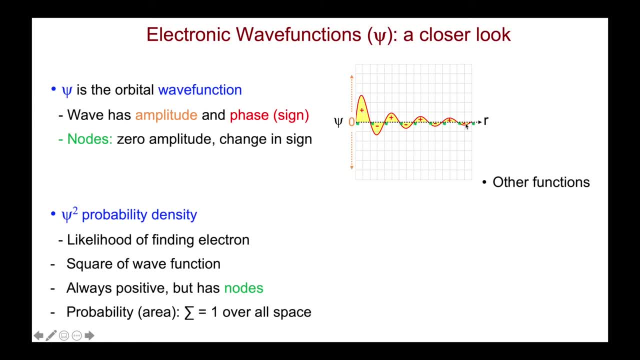 And in this case the amplitude just became zero. It becomes less and less with the distance r. This is psi squared for this particular function that I showed up here, Squaring it Same thing as the previous one. Now, psi squared is positive everywhere. That represents the probability. 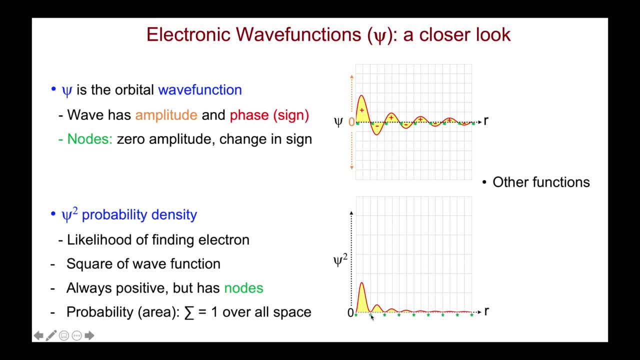 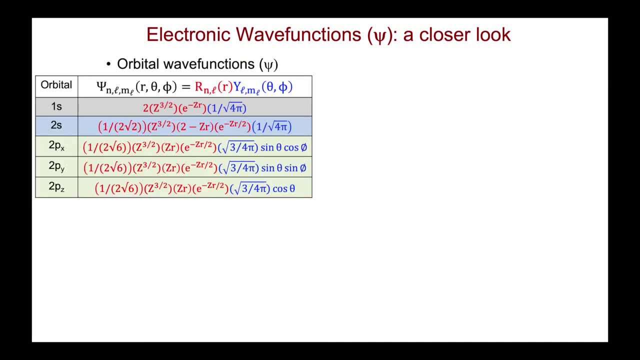 of the electron being in this particular place. We still retain the nodes where there is no probability. Our orbital wave functions deduced from quantum mechanics. they're a little bit dead-fit, more complicated, and I show them here for orbitals varying from the 1s through to the 2pc. 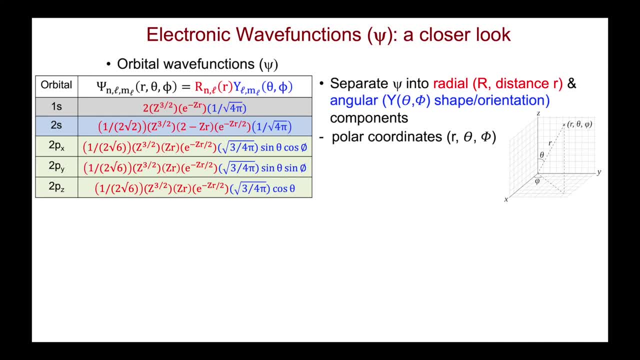 We can separate the wave function into two components. One is called the radial component. That is how the amplitude of the wave function varies as a function of distance from the nucleus, And we'll call this r. Then we also can separate it into an angular component. 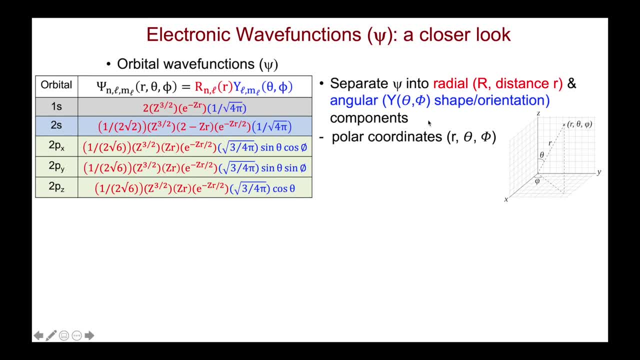 We call that y and this is how the amplitude changes with angle. So this would give us the shape and orientation of our orbital. As we separate into these two components, then we're using polar coordinates which comprise of distance and our two angles.